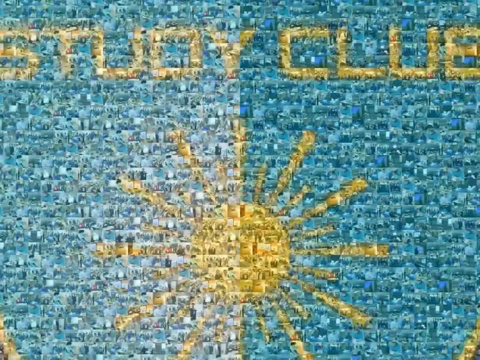 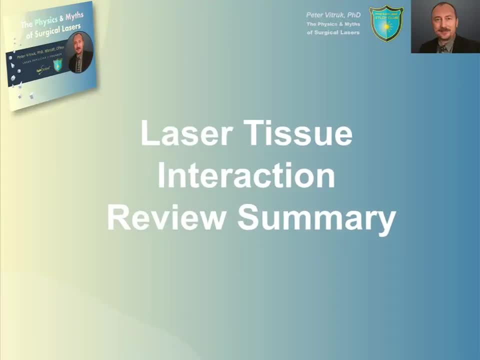 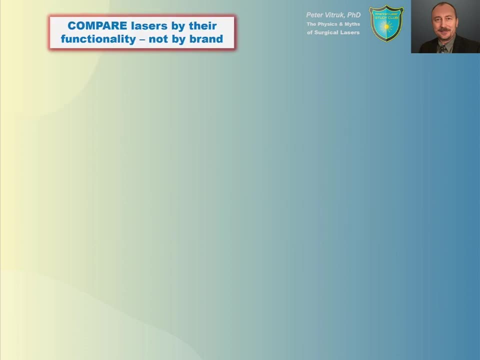 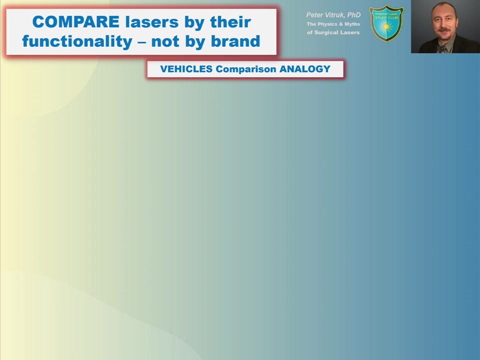 courses. Hello and welcome to this short review of laser-tissue interaction relevant for the soft-tissue surgical lasers. We want to look at the soft-tissue lasers from the perspective of their functionality. A very helpful analogy for us is the way we compare vehicles of different functionality. Take a look at the four. 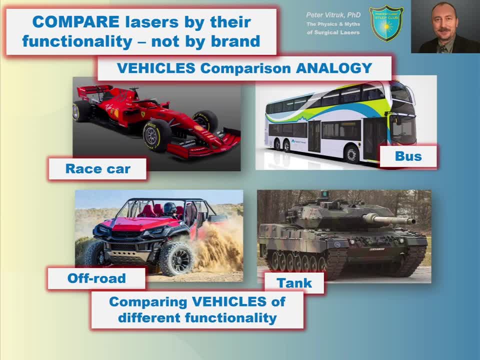 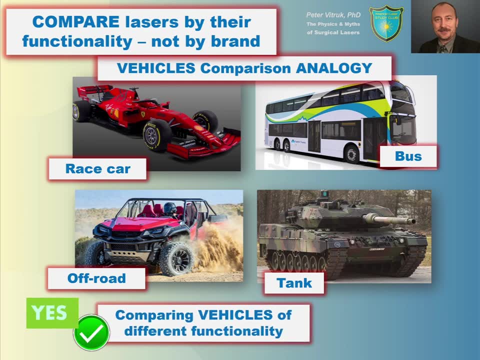 quadrants in this sketch. This is exactly the idea of how we want to look at the medical lasers out there as to what they can do functionally. So what defines a good soft-tissue surgical laser? The answer has two parts to it. 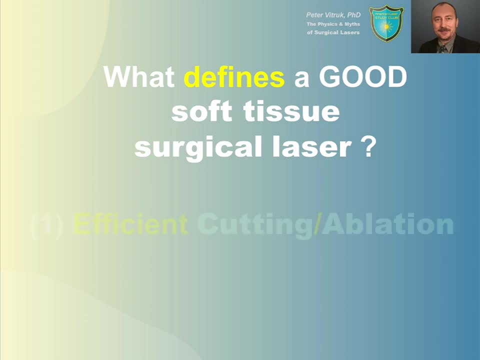 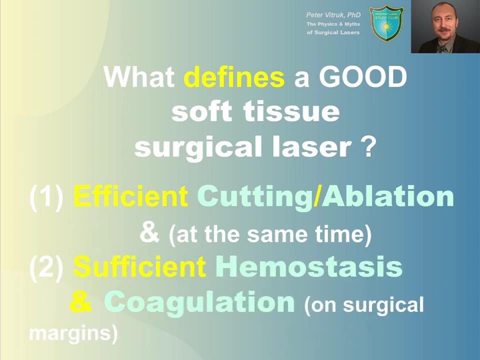 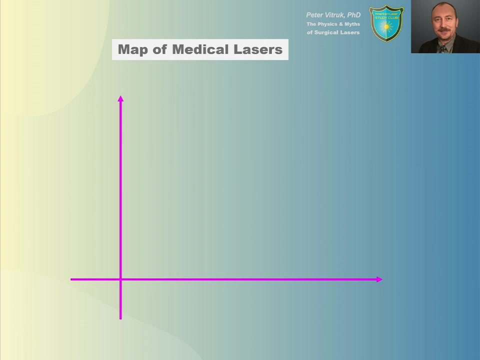 First, the laser beam has to be able to cut away, perize or ablate the tissue. Second, the laser beam has to provide coagulation and a hemostasis on a surgical margins. Pretty simple. So, since we now know that the kind of the laser, the 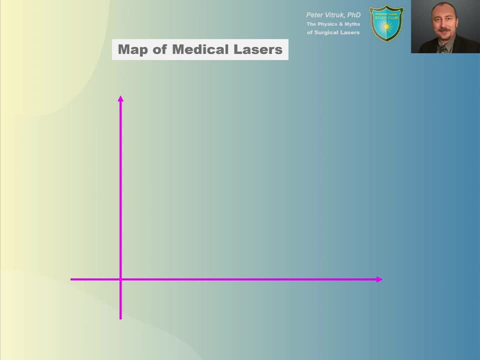 we want for the soft tissue surgeries has to cut and calculate at the same time. we just recognized that there are lasers out there that do not cut and do not calculate. here's a simple map of all lasers from the perspective of their ability to ablate and calculate: the top right corner. 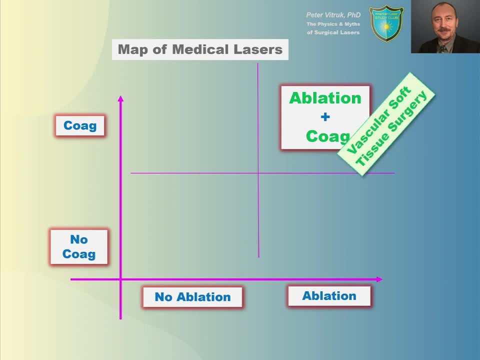 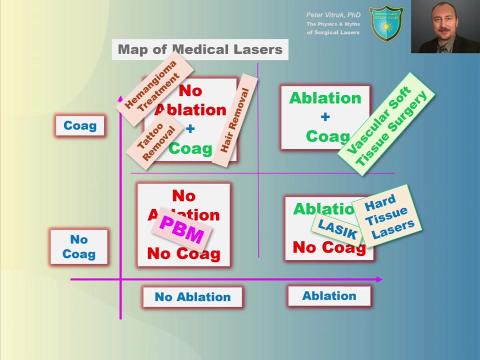 ablation and calculation, perfect for the vascular soft tissue surgery. another blade of laser, but with limited ability to calculate, perfect for these kind of applications. no ablation, but with the good cognitive properties. perfect for these kind of applications. and photo biomodulation is great use for the laser that does not inflict much of the thermal effects. so non-ablative lasers on. 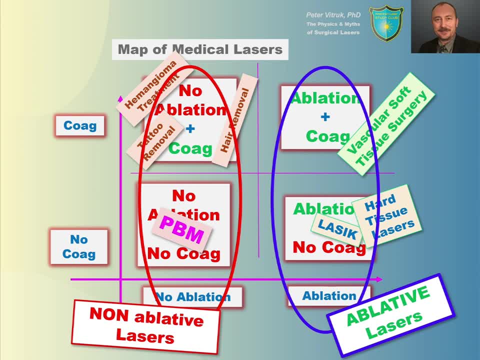 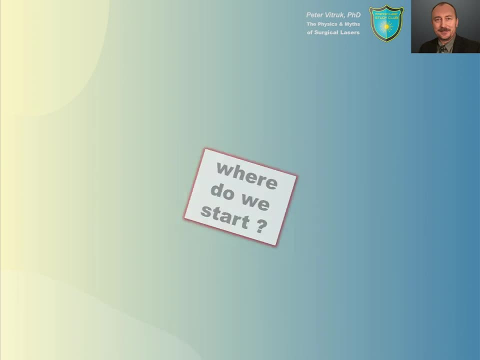 the right, i mean ablative lasers on the right, non-ablative lasers on the left. and here's a question which it is: specifically belong on the map, and where exactly on the map do they belong? to answer, we need to look at the physics of the laser tissue, interaction specific with the optical properties and more. 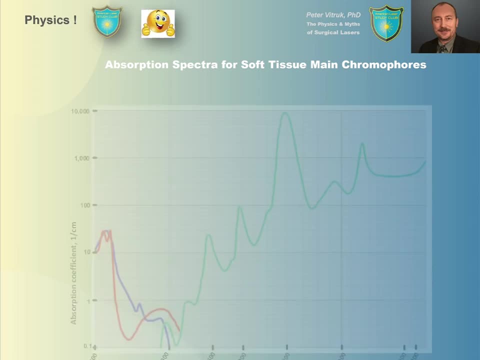 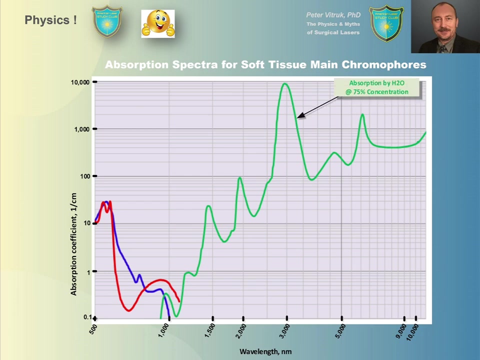 specifically the absorption spectra for the soft tissue main chromophores. here is the absorption spectrum for the water at the histologically relevant concentration of 75%. this is the hemoglobin- oxyhemoglobin at histologically relevant presence of blood in the soft tissue: 10%. now let's place the all of the diet and the new deeming young lasers on this chart. this is 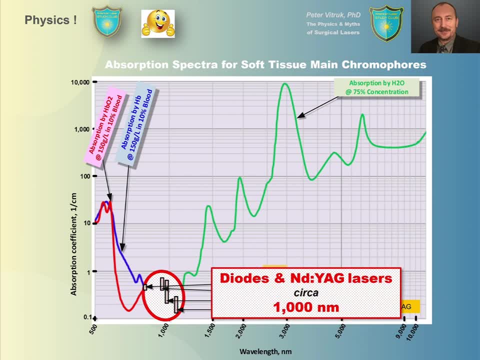 where they belong around 1,000 nanometers. notes the very low values of absorption coefficient, which means long distances, that's the. these wavelengths can penetrate through the soft tissue. all the CO2 lasers belong to the neighborhood of the 10,000 nanometers. that is strong absorption. 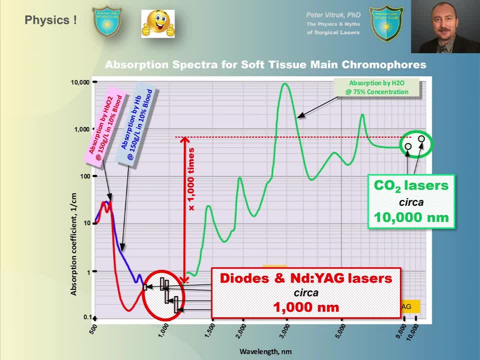 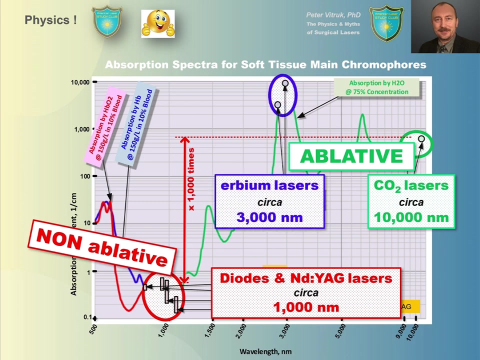 approximately thousand times stronger than for the diet and the new deeming young laser wavelengths, which means that this explains the why the diets and the new deeming young lasers are referred to as a non ablator with CO2. lasers are ablates and so they were. 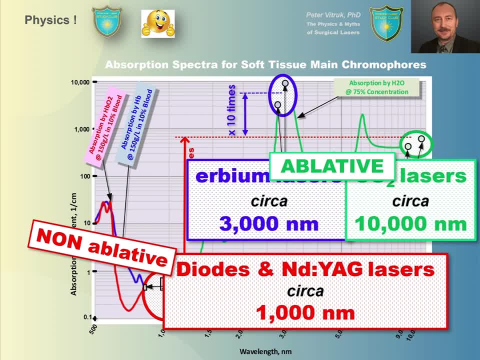 blade that a laser is. line blanks classes and one of знает it bear. my laser is characterized by the ulenoto calculation, just because of them, very shallow depth of penetration of those wavelengths into the soft tissue due to very strong absorption, the diodes and the neodymium yaks, they're characterized by very deep coagulation, just. 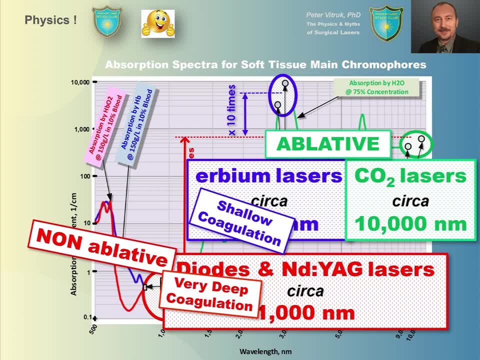 because of the very weak absorption these these wavelengths can go to the soft tissue for the long distances the co2 laser is in between those two classes as far as the depth of the coagulation, and in fact it's an optimal wavelength for coagulating sub 50 vessel diameters. so summary: 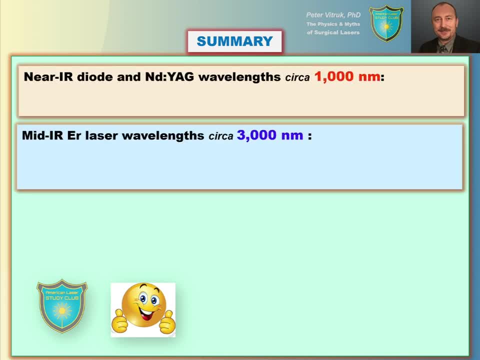 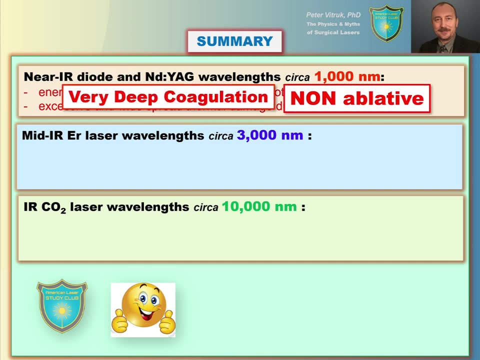 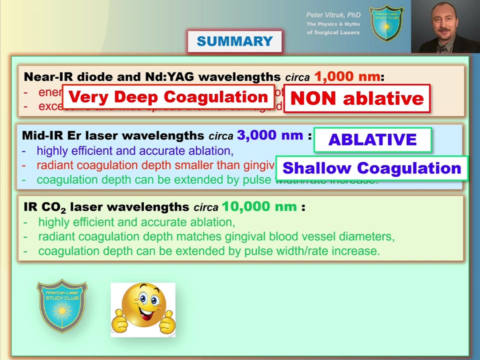 is for the a thousand three thousand ten thousand nanometer class uh wavelengths. one thousand nanometer, non-ablative with perfect deep coagulation, three thousand class, three thousand nanometer class devices, perfect ablative devices, but was limited depth of the coagulation. the co2 lasers are not your best colors, not the best calculators. 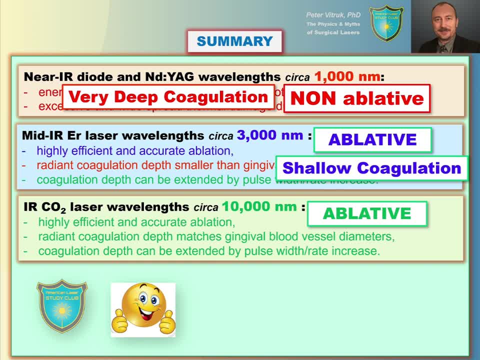 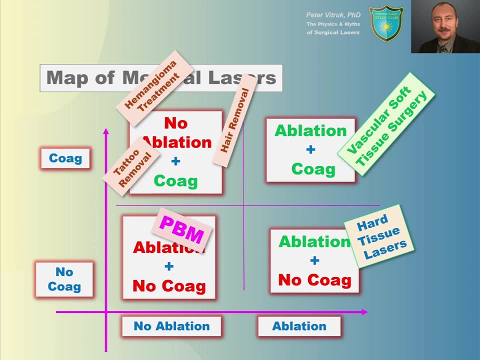 but they do this at the same time efficiently and the optimal for the sub 50 micrometer blood vessel diameter calculation. right back to our map of the ablative coagulative laser classes. co2 laser fits the bill for the vascular soft tissue surgery. erbium lasers fit the bill nicely for the heart. 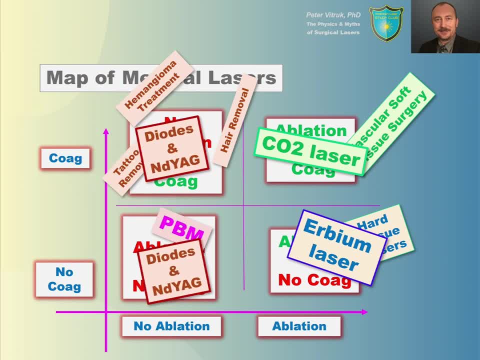 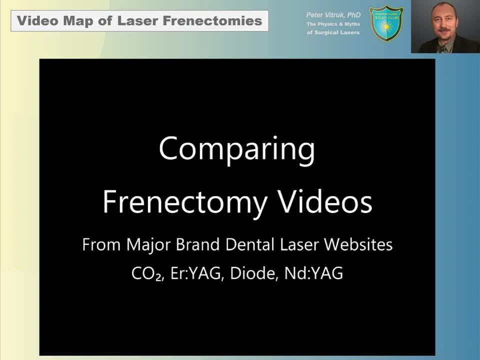 tissue and diets and the needing yaks fit the bill for the non-ablative applications. so now let's look at the several videos, which are organized, arranged similar to the map of our medical lasers in the previous slide. all four videos are taken from the public domain on youtube. 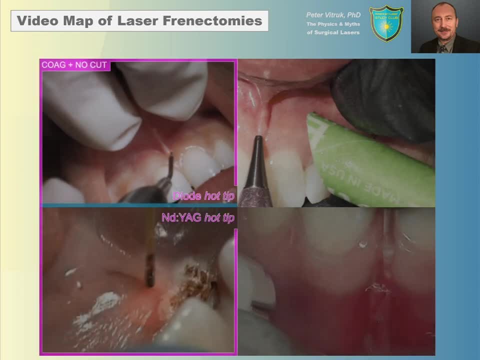 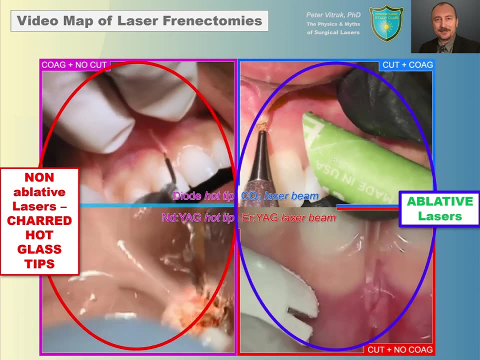 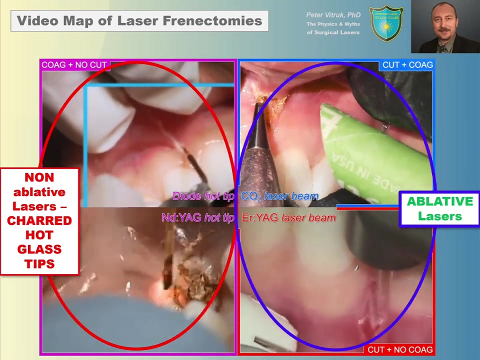 these are build. this will be the uh lip type of an actinys: ablative on our right, non-ablative on the left, uh on our left. we have the non-emblatable lasers turned into the hot tip cutter devices by turning them into the chart hot glass tips top right corner. fast and bloodless. 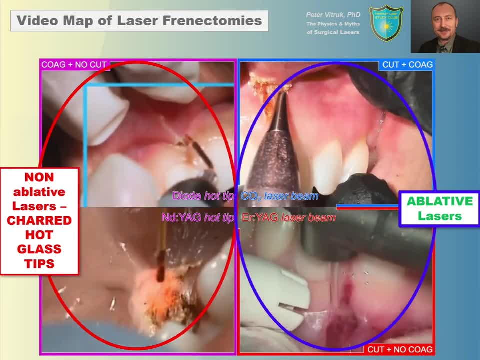 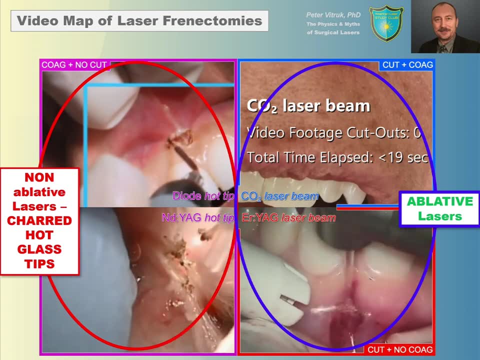 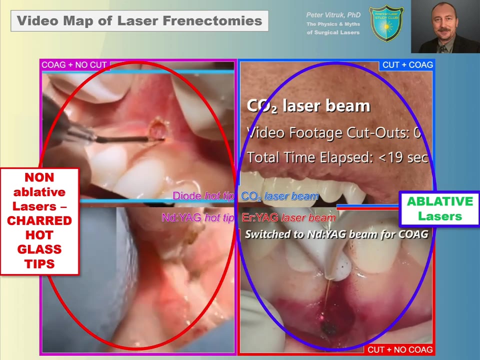 pseudias of an acting: top left, slow, hot tip. rotary. bottom left- painful to watch. hot tip. bottom right, fast, bloodless incision, but the blood is simply washed away by the powerful water spray. Now switching to a different handpiece with a different wavelength: now it's a neodymium. 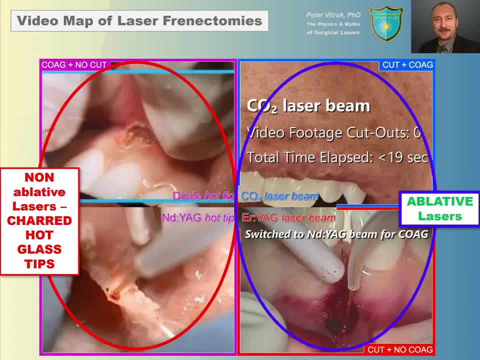 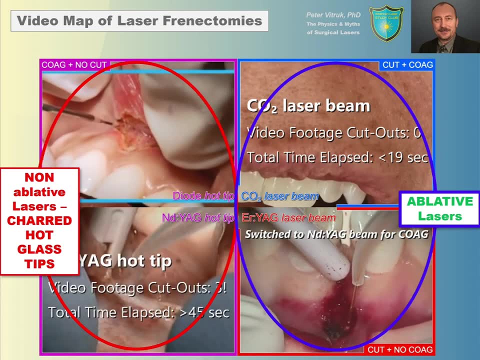 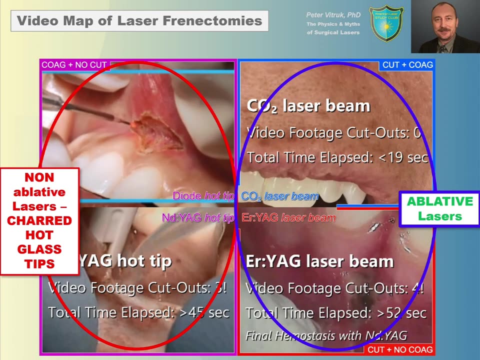 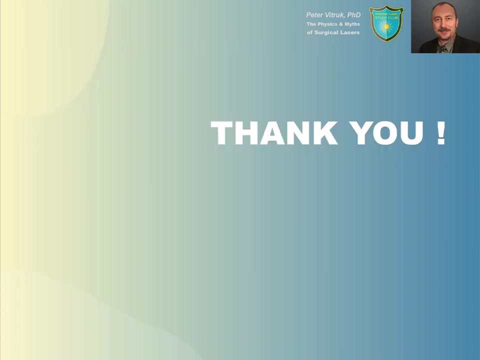 YAG that calculates the pool of blood, Not exactly the best way to use the surgical laser. The CO2 laser was the fastest and the other three devices took three to four times as long as the CO2 to complete the lip phrenectomy. I thank you for the time you took to watch.